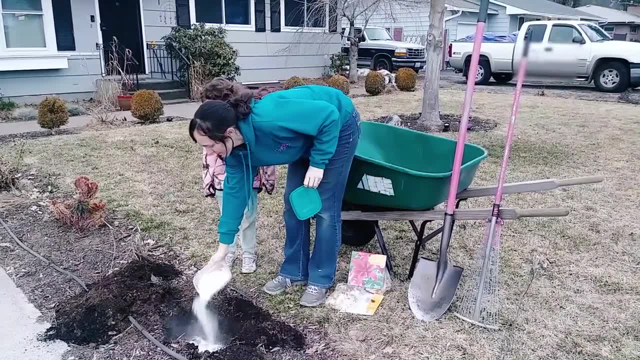 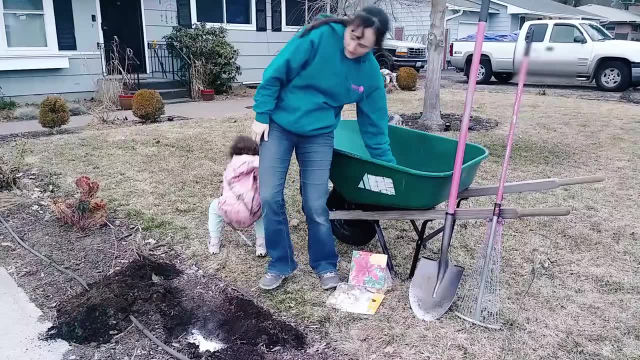 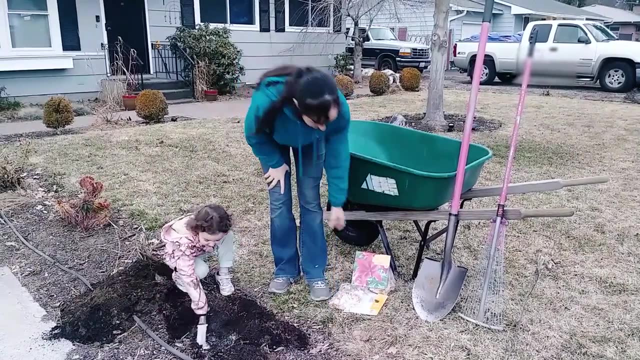 We're just going to sprinkle it in Tap And then we'll stir it up a little bit. Where's your hori hori? Can you stir up the soil? Stir, stir, stir. It's almost like baking a cake, Almost, But with oil, But with oil. 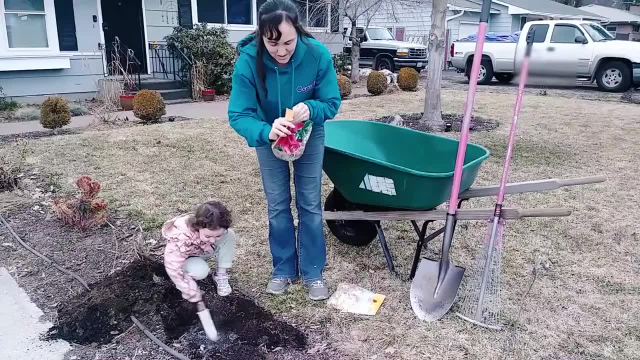 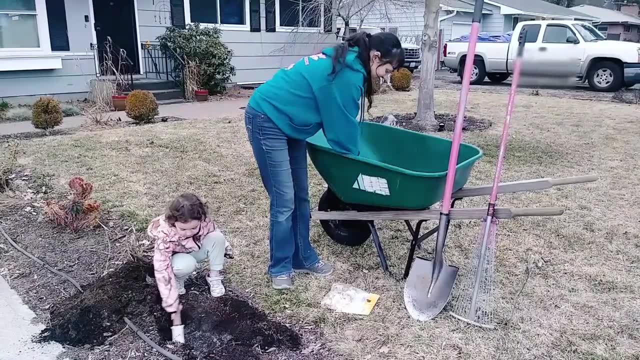 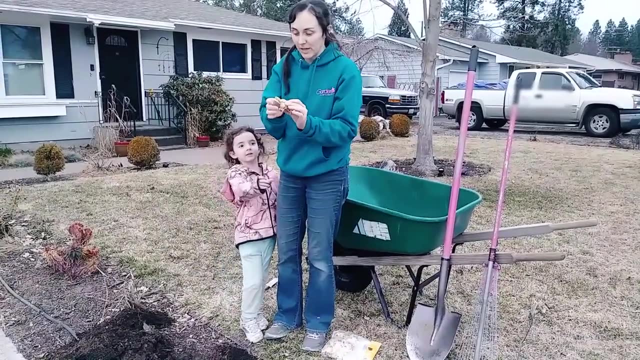 But with plants, But with plants, Okay. So most summer bulbs you can plant as soon as the all danger of deep frost is past. These ones are starting to grow already, so it was getting kind of urgent, Otherwise it would get a little bit early in the season. 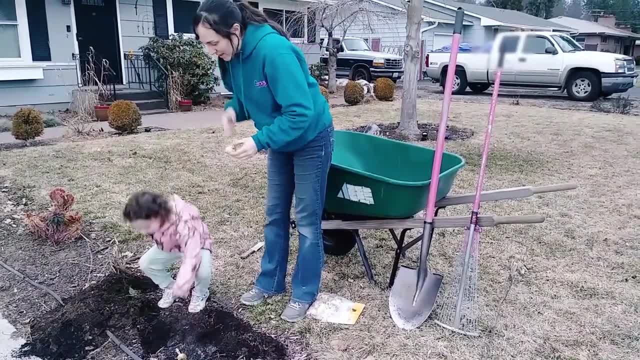 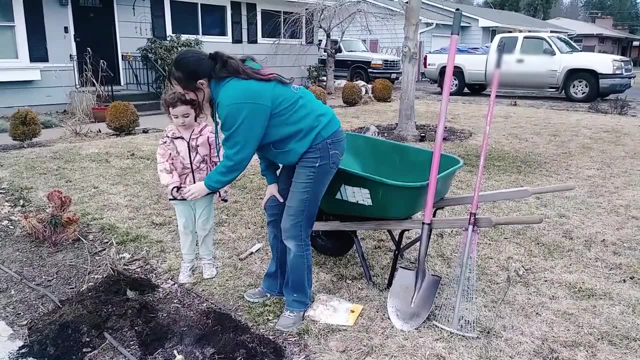 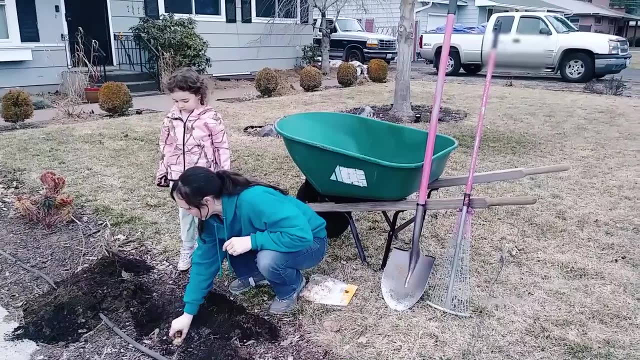 But I wanted to get them into the ground Now. good job, This is up Roots, Roots are down. Put them in the hole Now. you don't want it on your side. You want it pointing up, Reaching for the sky. Reach for the sky. 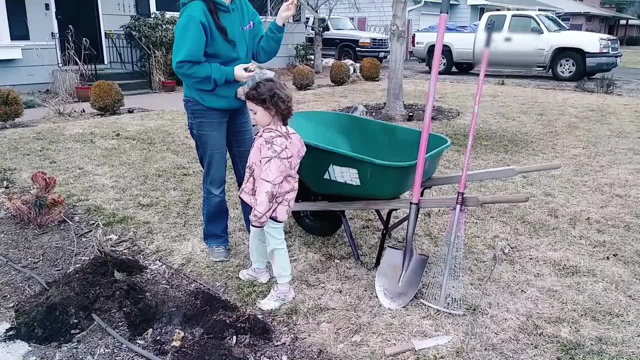 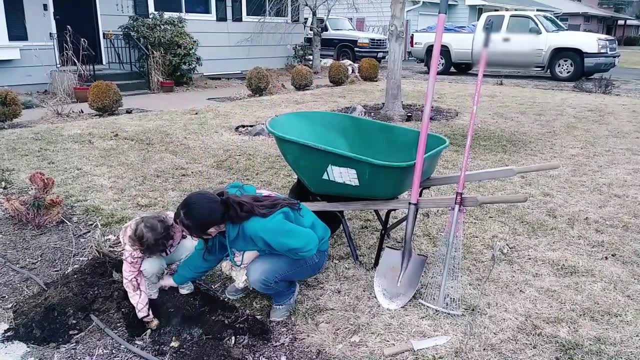 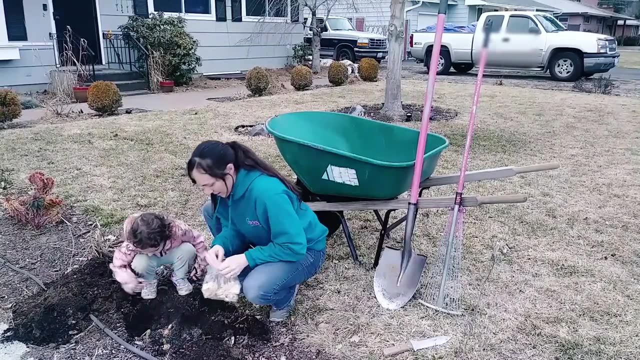 Depth is eight inches. Spacing is three bulbs per square foot, Three. So, yeah, about three to four inches apart. Good job, Okay, We're going to put that in the middle. We're going to put this one kind of up here And then put one more. 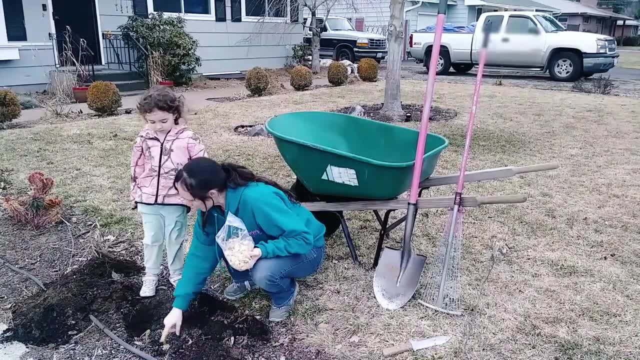 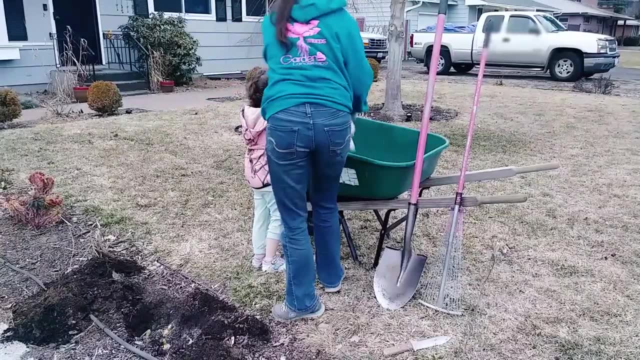 These are the black ones over here. That's right. So it's like a domino or an X Yep. Okay, Now we're going to fill this hole back in. Can you help me fill the hole back in? Use your hori hori. Use your hori hori. 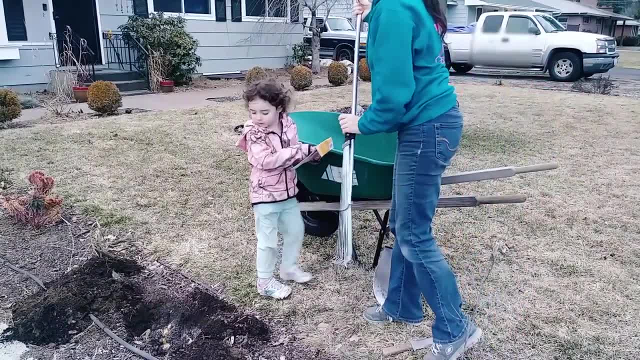 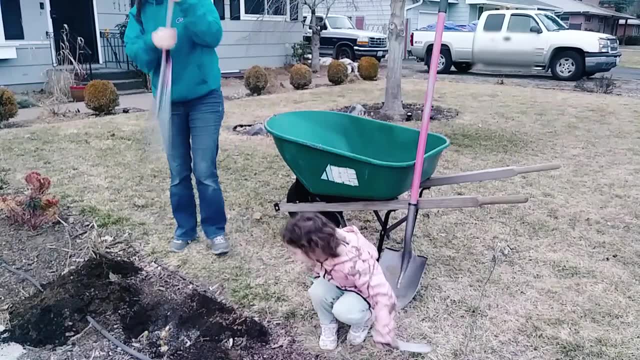 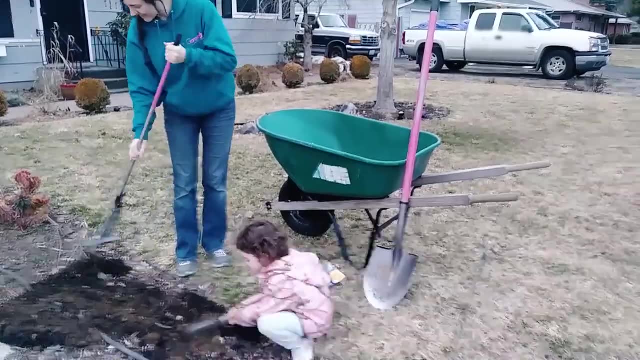 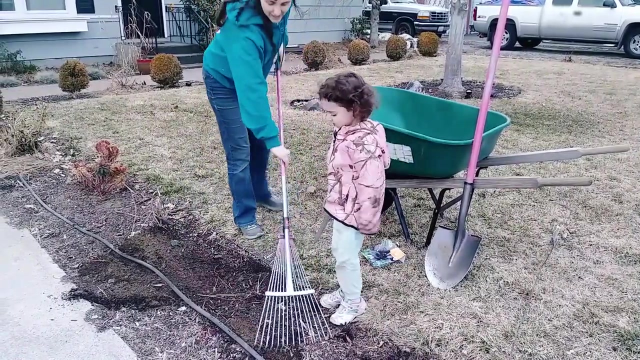 One, two. next step: Dig it in. Dig it in. She said: Where's my hori hori? I've got it above my hori hori. Gently move the soil back on, Break your garden area, just like that. 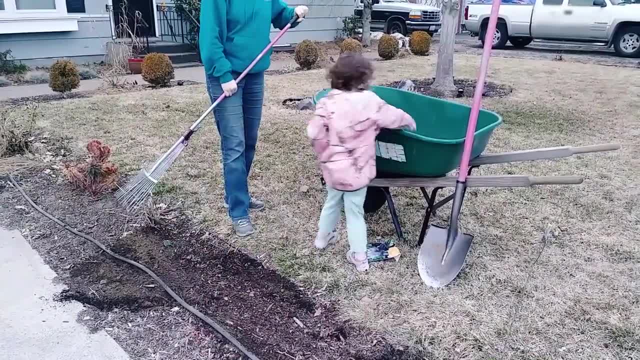 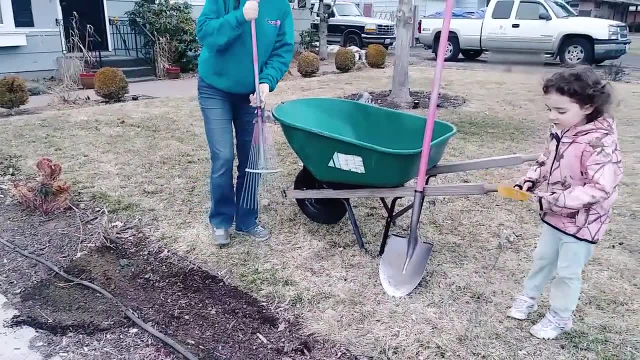 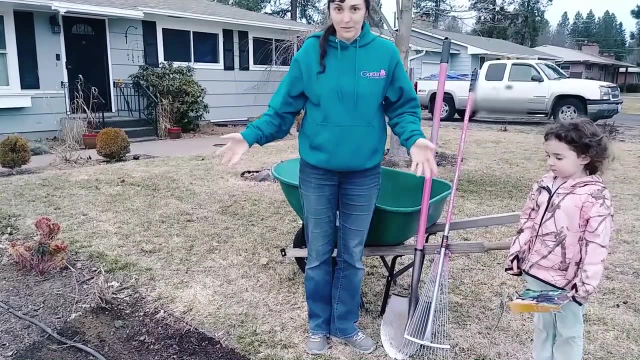 And that is how we plant lilies. And step three: Wait and dig the other one, Wait and dig the other one. Now we can also water this in. We're not going to today because it's still just a little bit cold And I honestly haven't turned my water on yet.